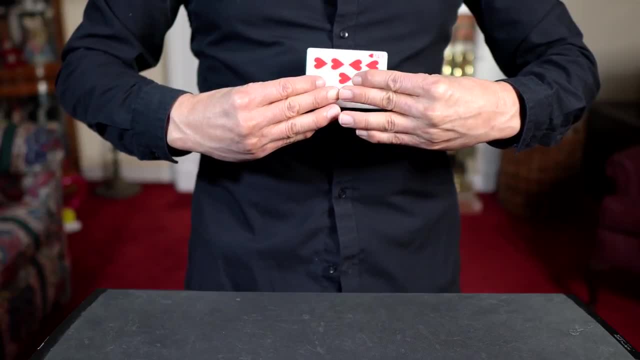 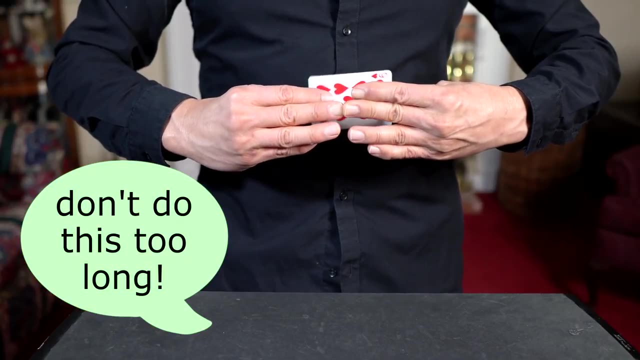 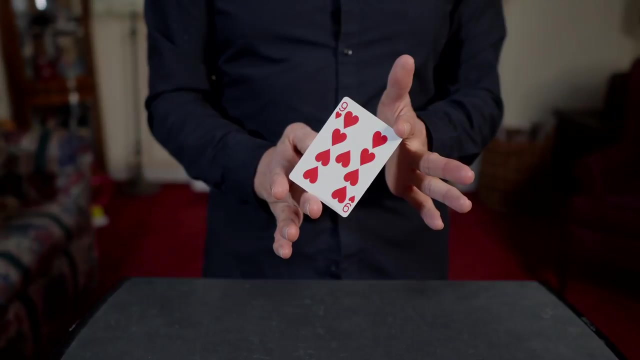 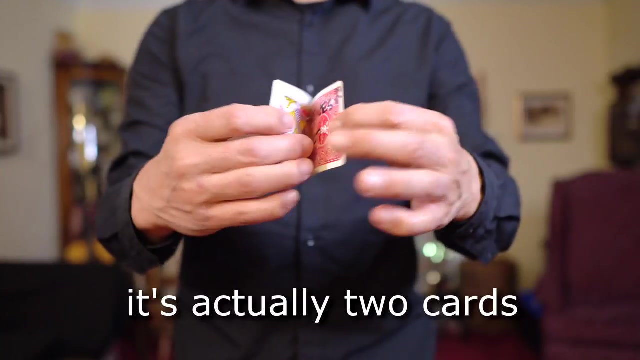 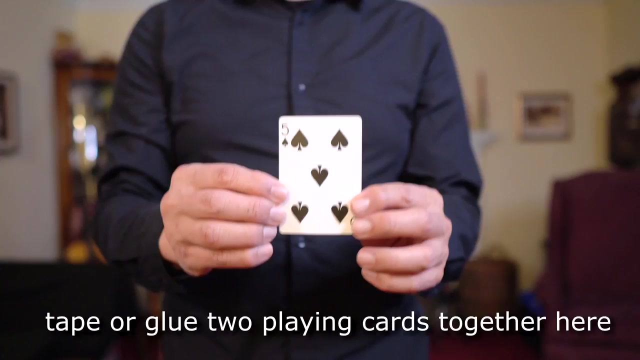 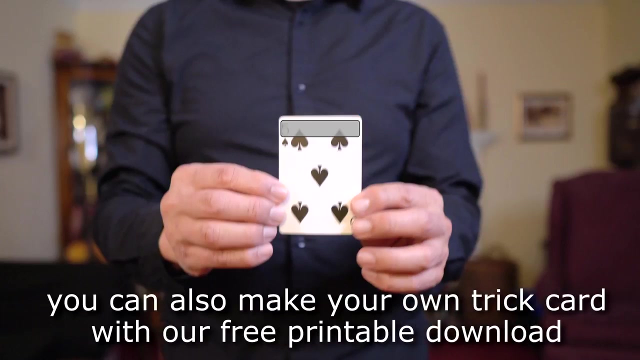 Your thumbs. grab the edge, fingertips, touch and just move your thumbs around, Just like this. Don't do it very long, You just want spectators to react. Grab the card and show it to be absolutely normal And you're in aed formed. 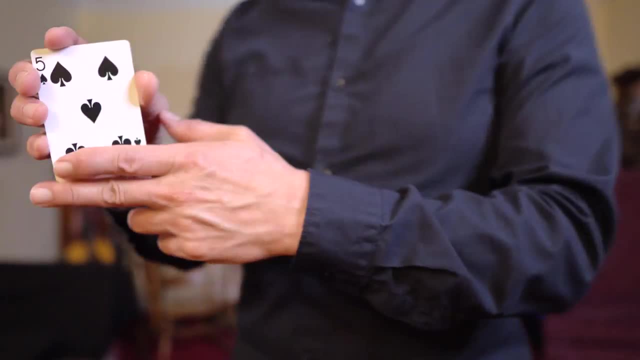 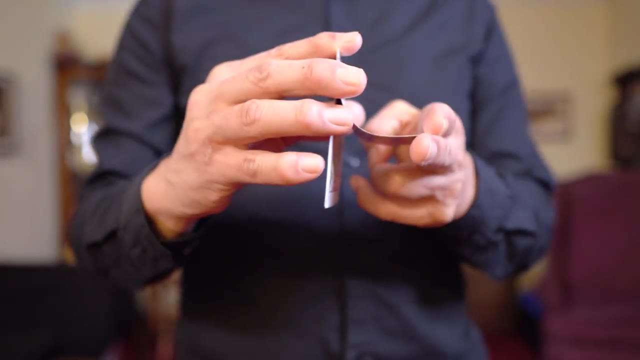 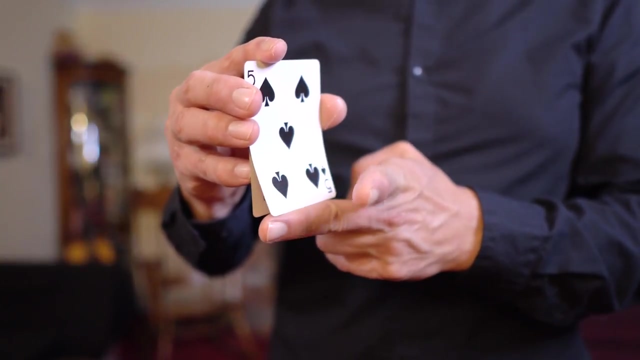 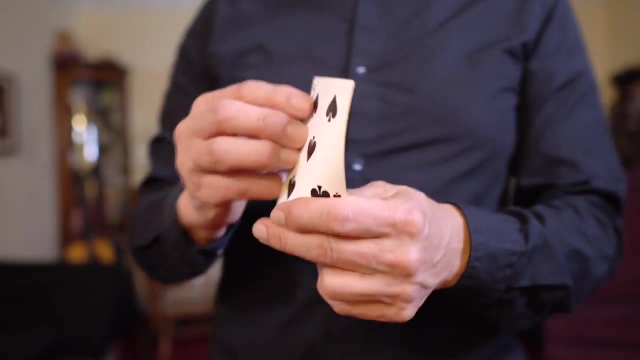 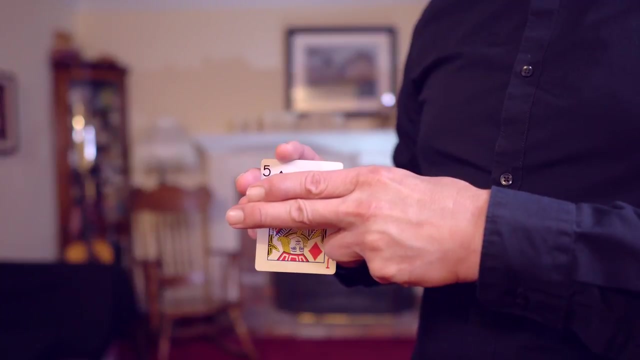 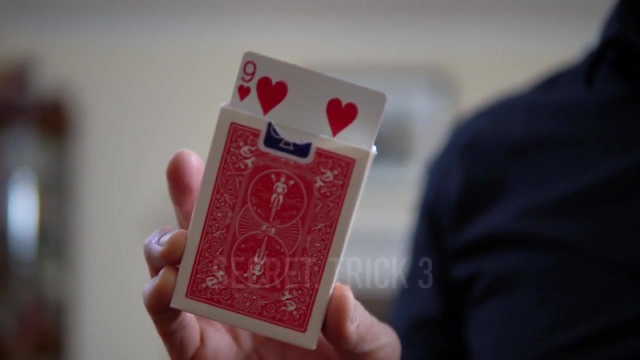 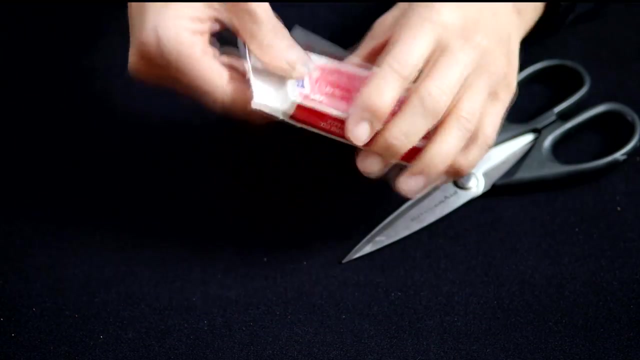 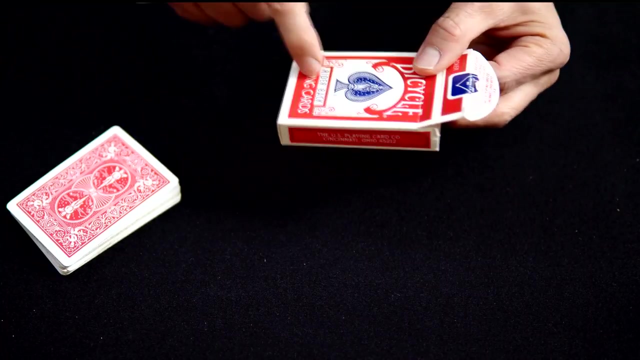 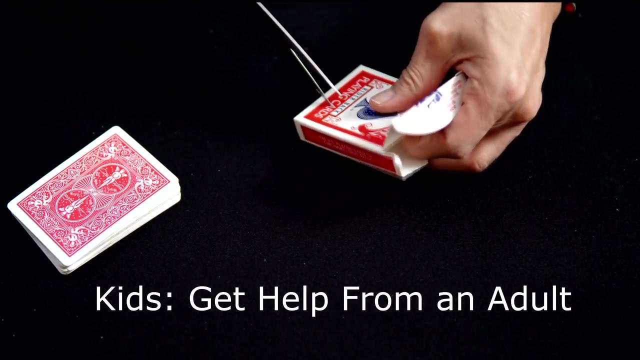 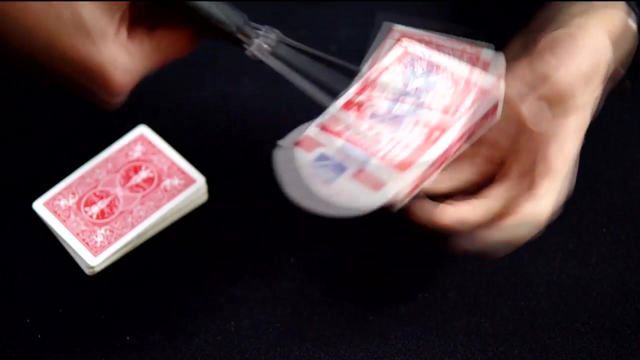 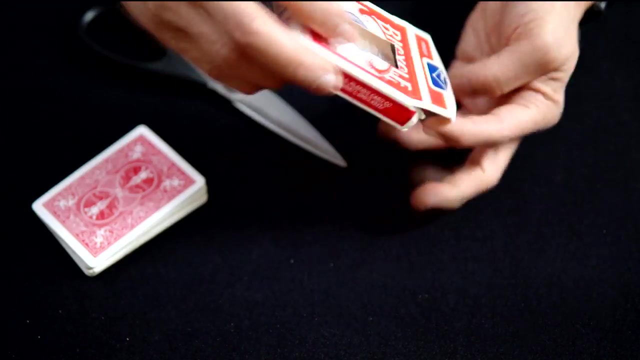 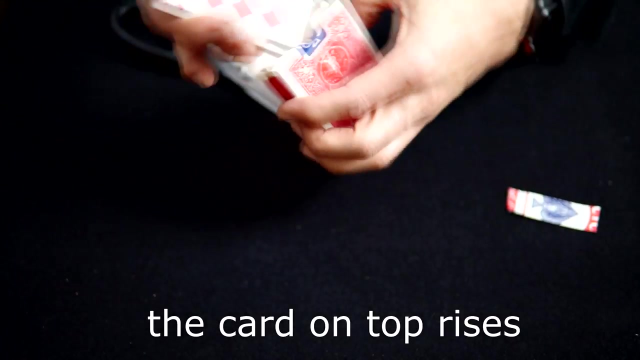 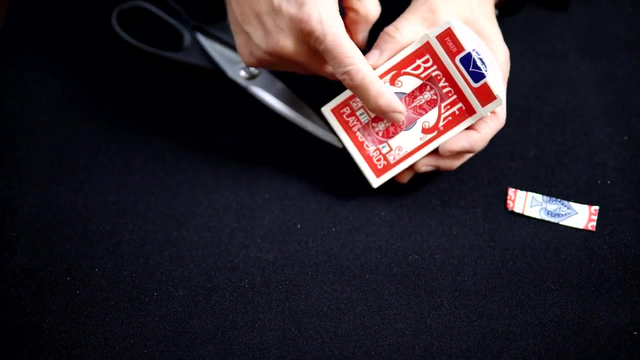 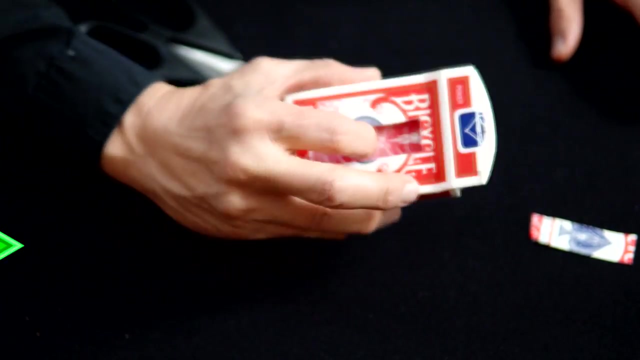 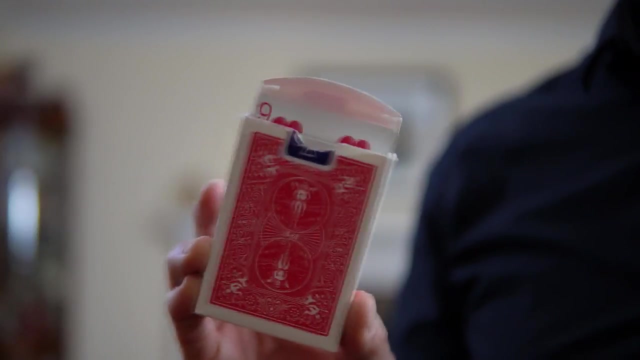 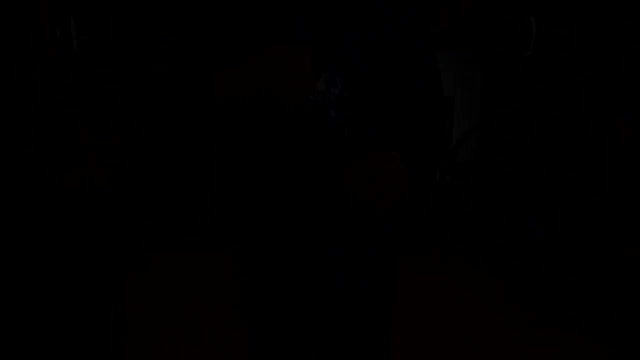 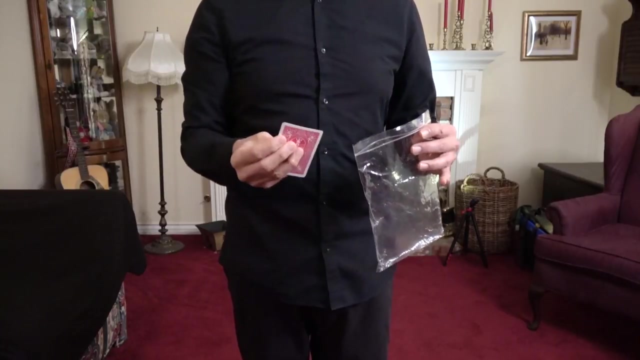 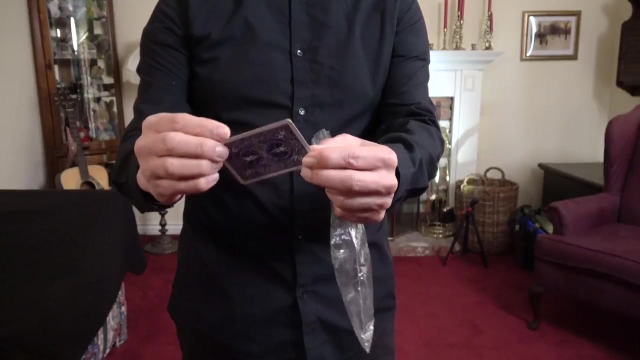 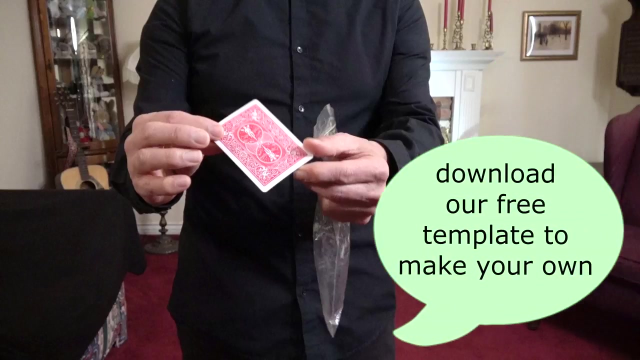 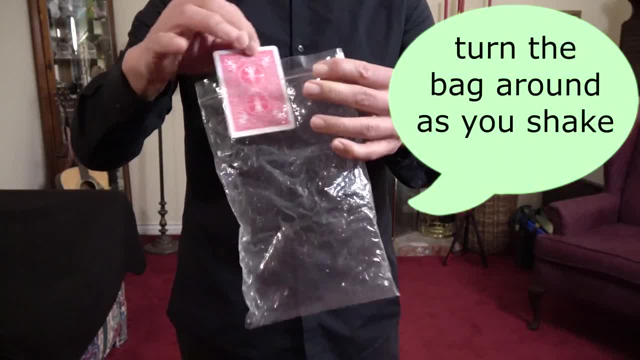 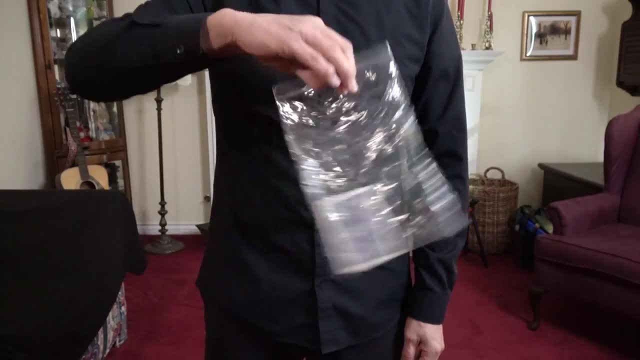 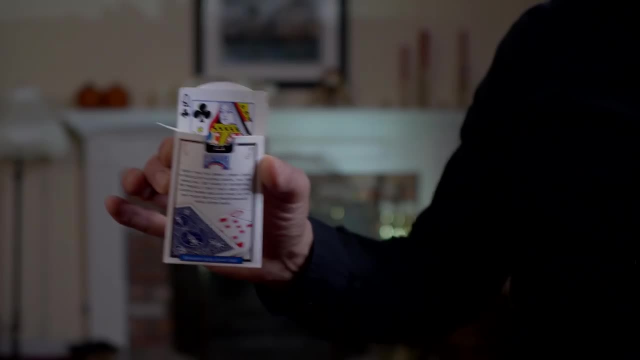 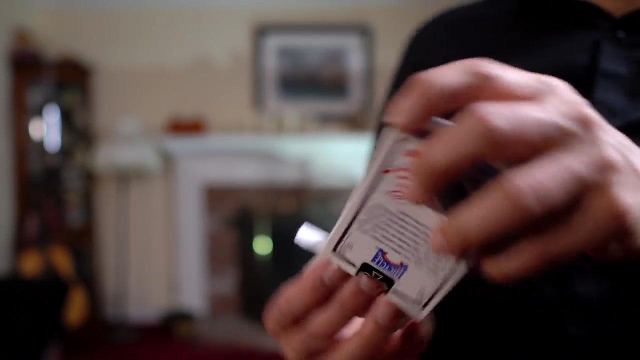 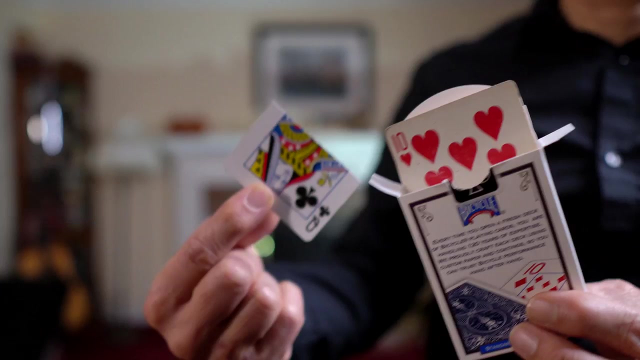 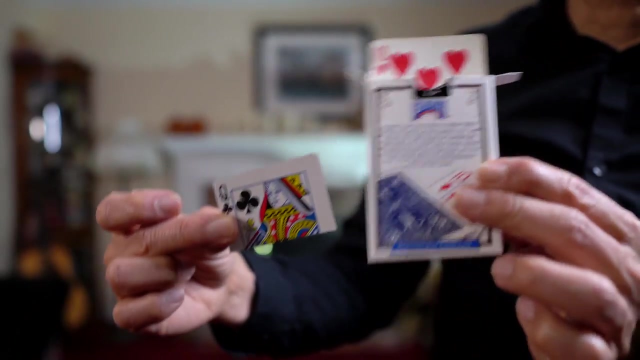 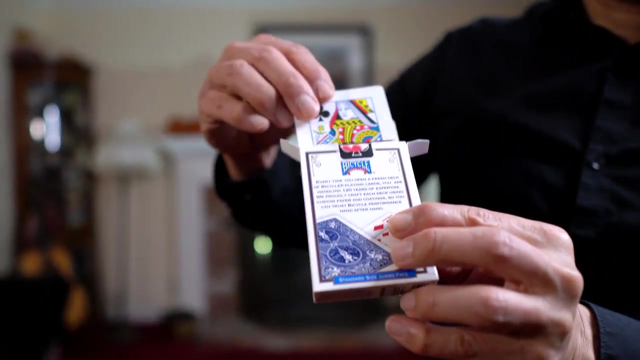 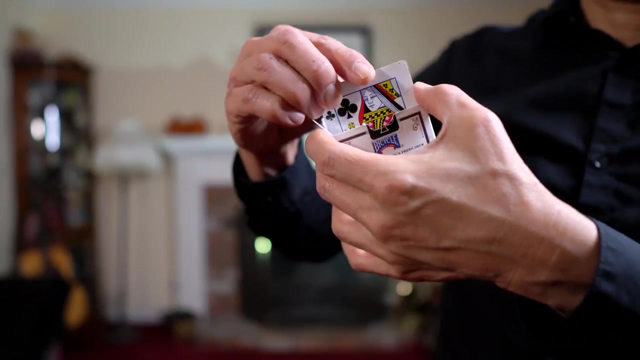 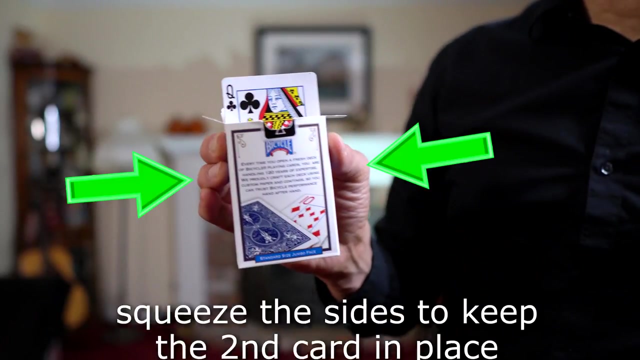 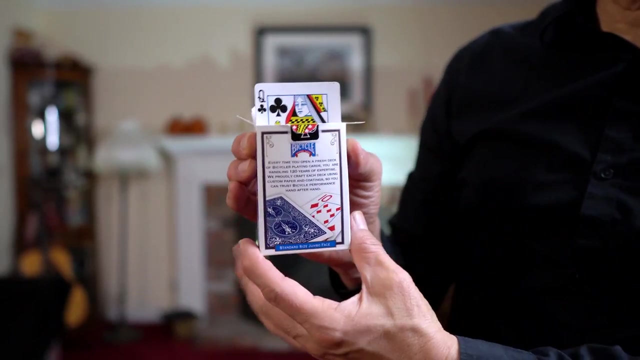 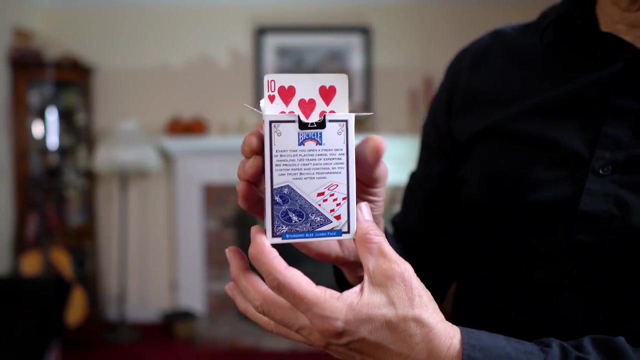 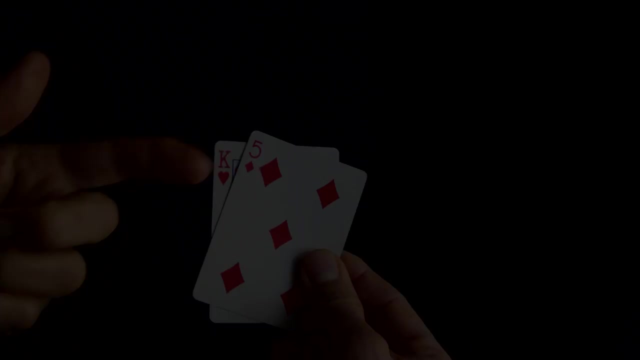 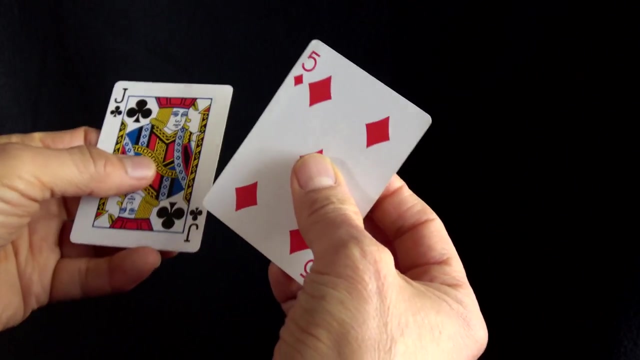 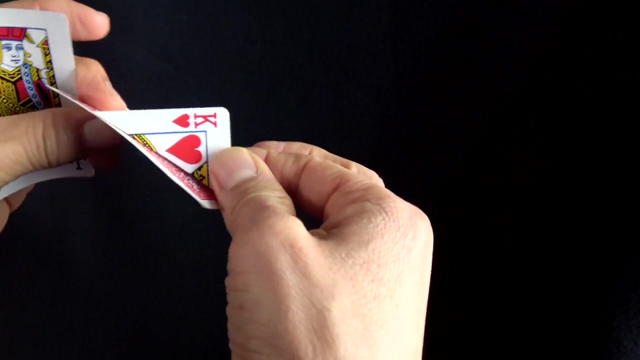 We'll be right back. We'll be right back, We'll be right back. Here's how the change works. You're going to create a gimmick card. This one's normal. This one is not normal. You've taken a corner from another playing card. 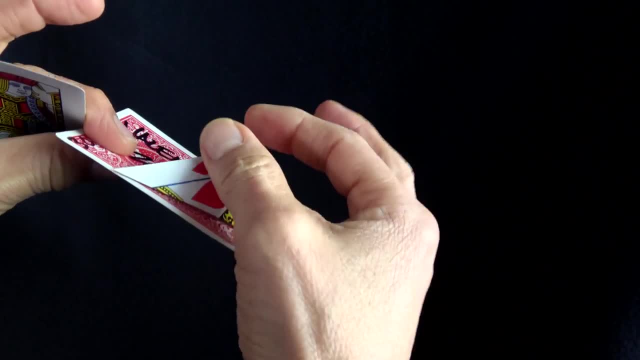 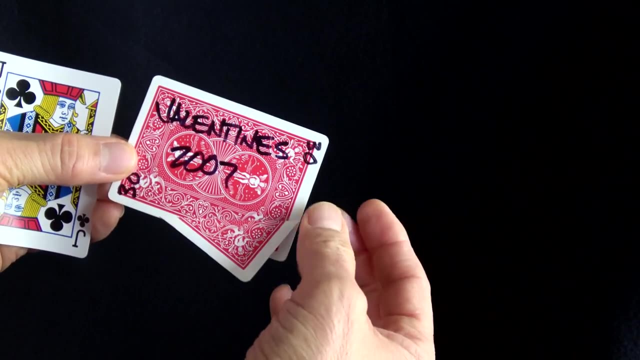 and taped it on right here. So you have this flap. It's just one corner from another card. Sorry about this. I've just been using old cards for these things, So that's Valentine's Day 2007.. Some magic event I did. 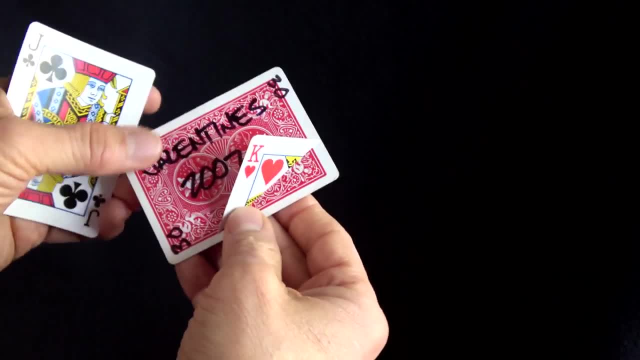 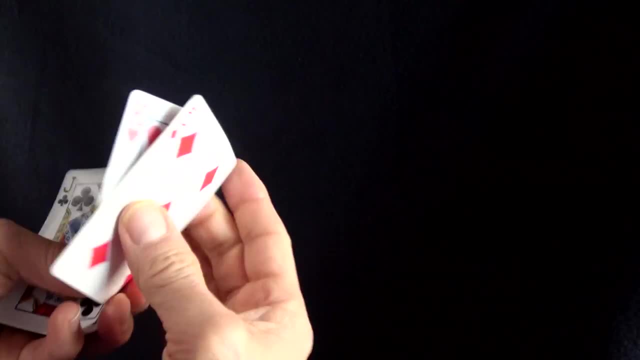 and I have no idea what it's from. anyway, A little side note there: Just use whatever playing card you have, Cut a corner off, Tape it right here, so you have this flap that moves And you're ready to begin the trick. 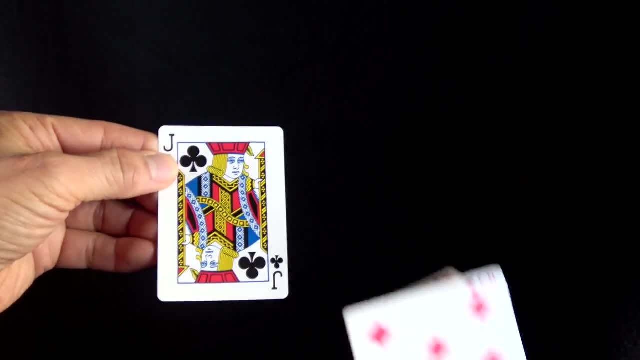 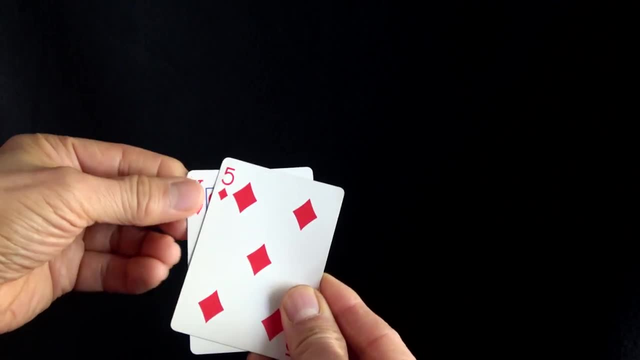 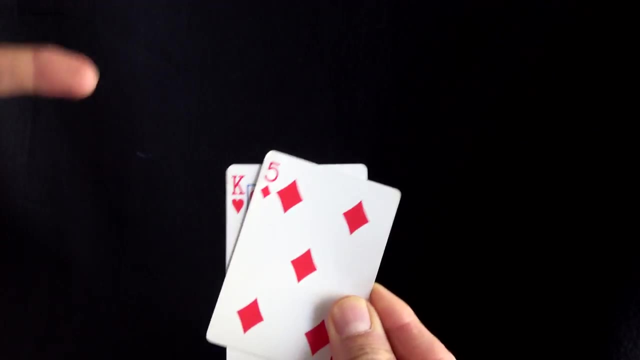 What you do is line up the bottom card. The bottom card is the second card that it will change into. Line them up as best you can. Now, with this finger, you're going to kind of flip down and to the right. So down and to the right. 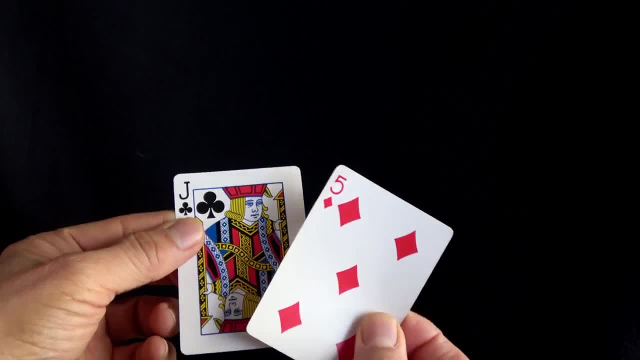 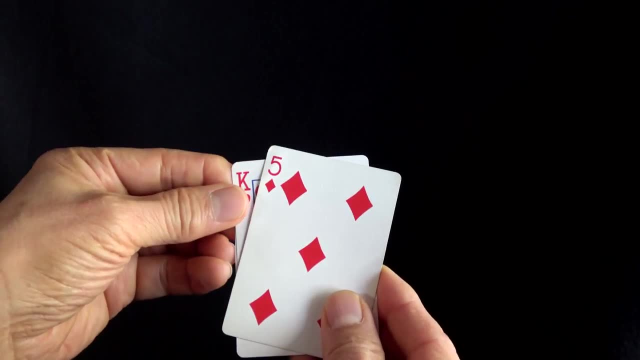 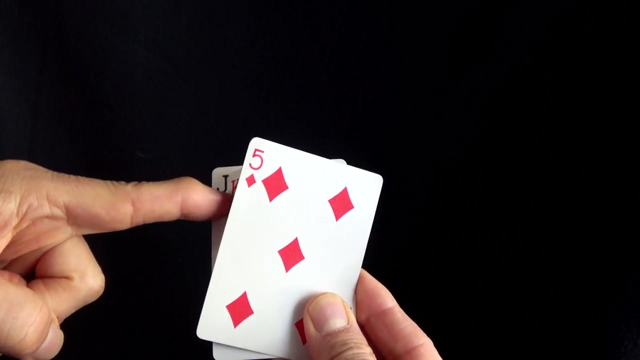 And then the spring action of this card tends to make this pop back up and lock in over here. Let's see if I can do this in slow motion. So I just take my finger like I'm pointing and then I push.